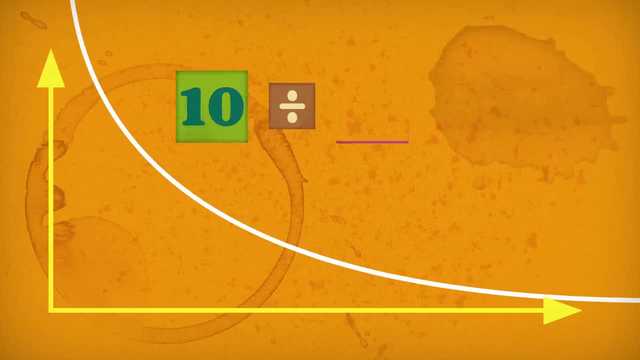 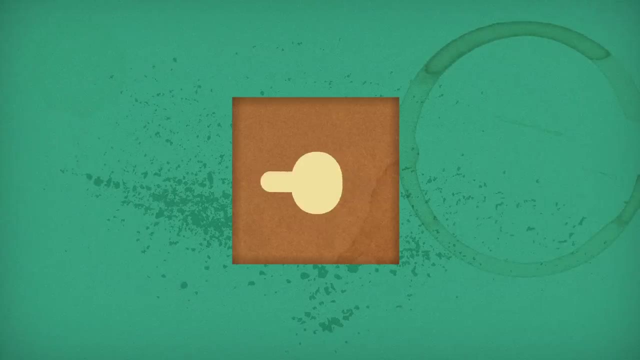 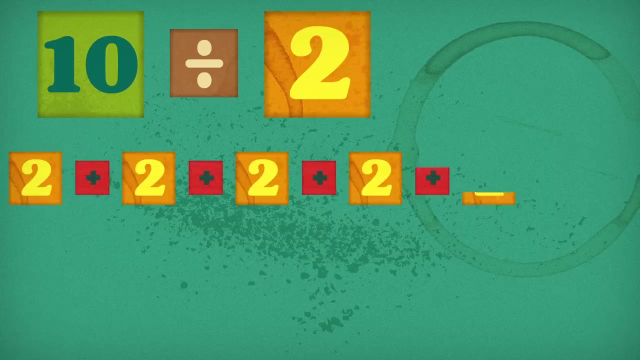 And that's not the same thing as saying that 10 divided by zero is equal to infinity. Why not? Well, let's take a closer look at what division really means. 10 divided by 2 could mean: how many times must we add 2 together to make 10,? 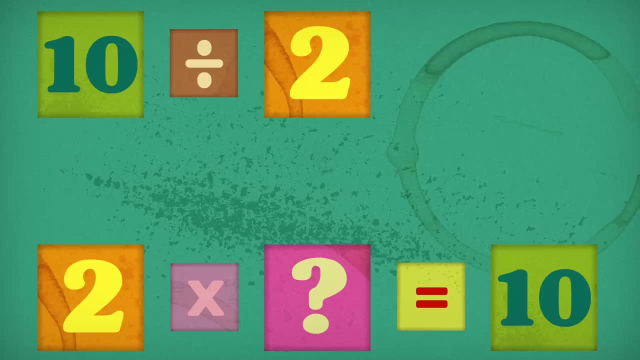 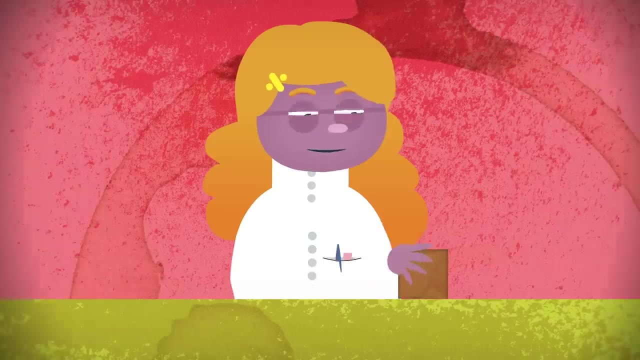 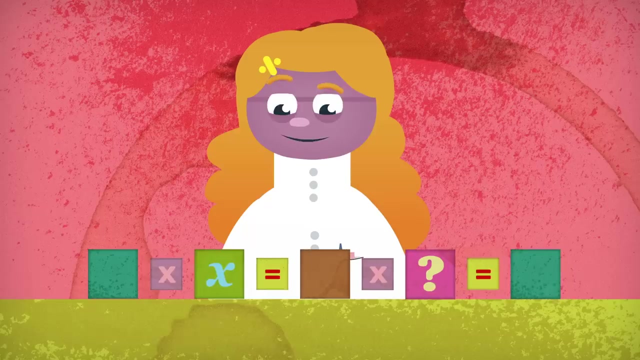 or 2 times 1.. What equals 10?? Dividing by a number is essentially the reverse of multiplying by it, in the following way: If we multiply any number by a given number, x, we can ask. if there's a new number, we can multiply by afterwards to get back to where we started. 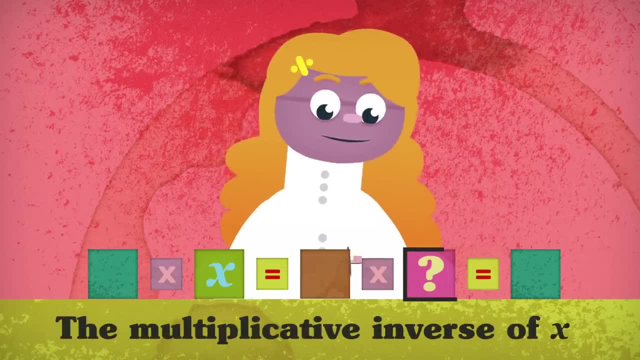 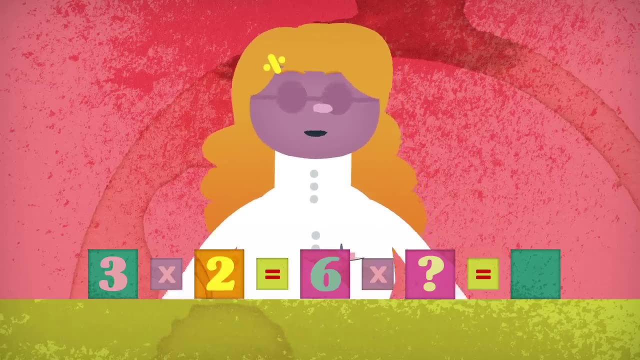 If there is, the new number is called the multiplicative inverse of x. For example, if you multiply 3 by 2 to get 6, you can then multiply by 1 half to get 2.. If you multiply by 1 half to get 2,. 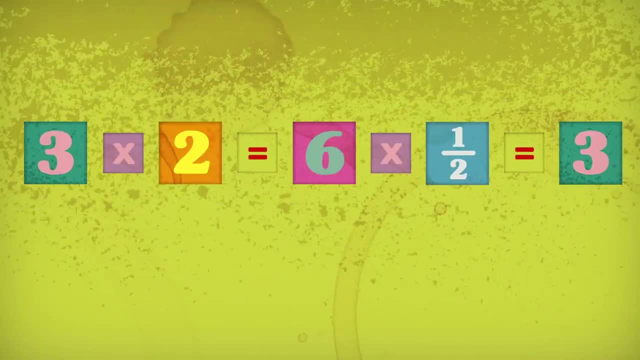 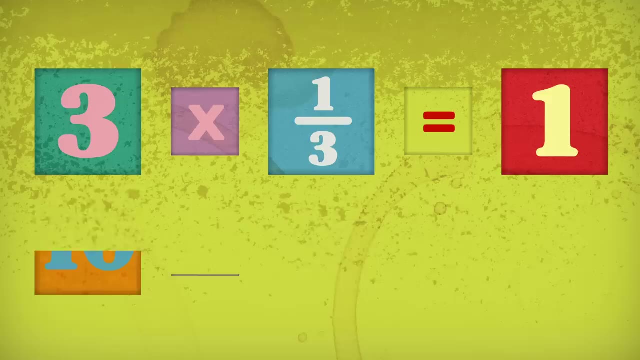 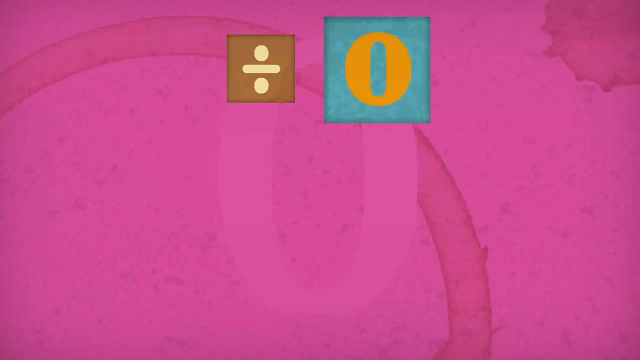 you can then multiply by 1 half to get 3.. So the multiplicative inverse of 2 is 1 half and the multiplicative inverse of 10 is 1 tenth. As you might notice, the product of any number and its multiplicative inverse is always 1.. 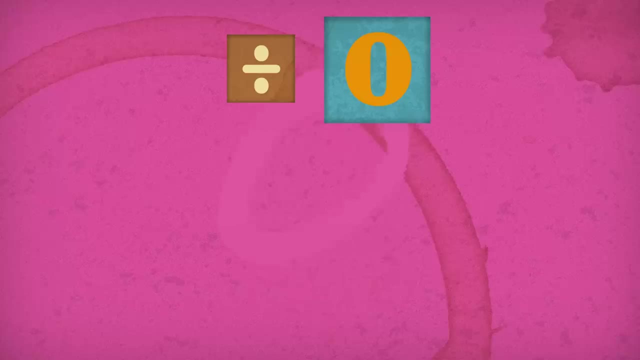 If we want to divide by zero, we need to find its multiplicative inverse, which should be 1 over 0. This would have to be such a number that multiplying it by zero would give us the same number: give 1.. 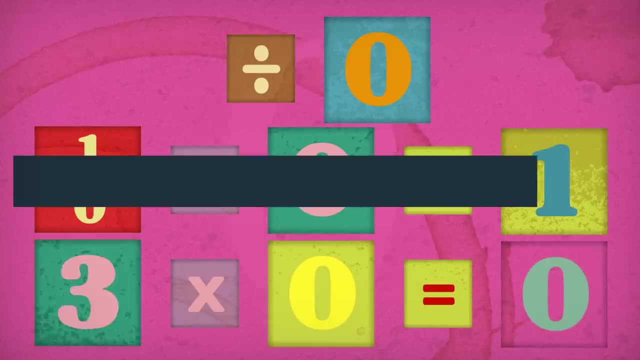 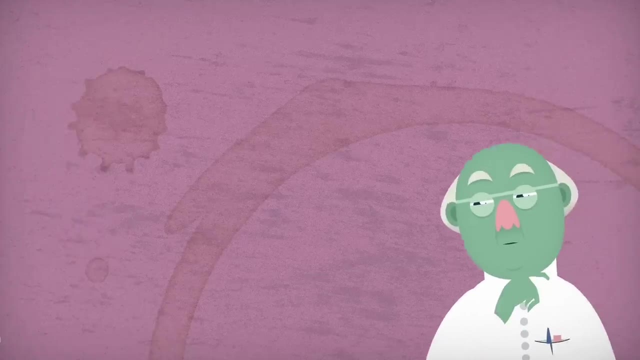 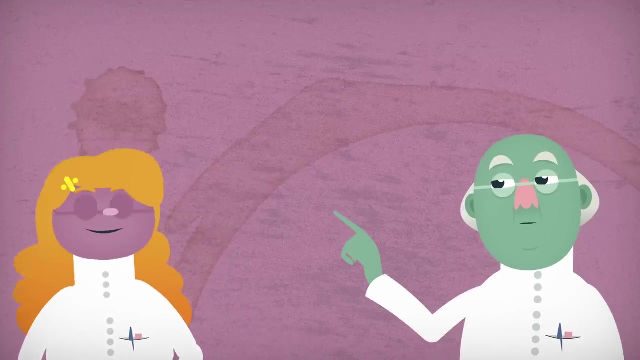 But because anything multiplied by 0 is still 0, such a number is impossible, so 0 has no multiplicative inverse. Does that really settle things, though? After all, mathematicians have broken rules before. For example, for a long time there was no such thing as taking the square root of negative. 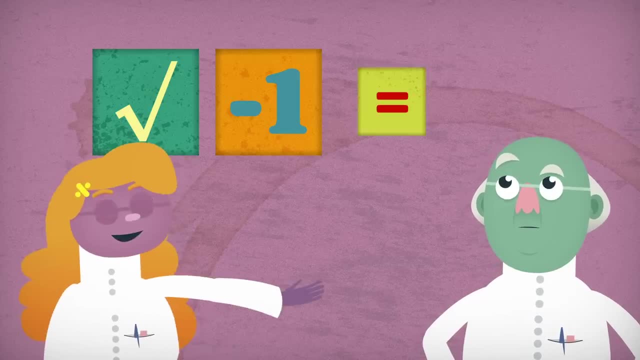 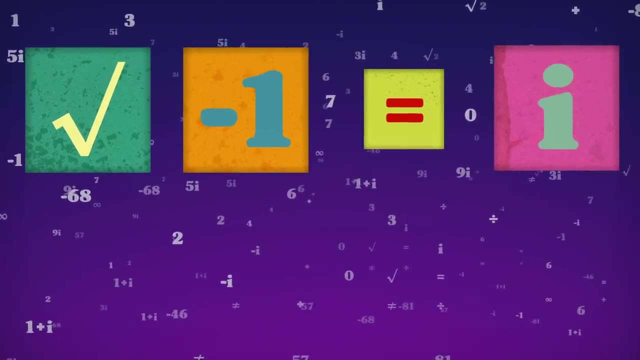 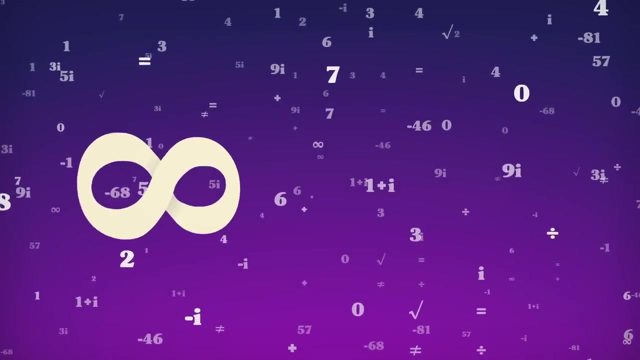 numbers. But then mathematicians defined the square root of negative 1 as a new number called i, opening up a whole new mathematical world of complex numbers. So if they can do that, couldn't we just make up a new rule, Say that the symbol infinity means 1 over 0, and see what happens. 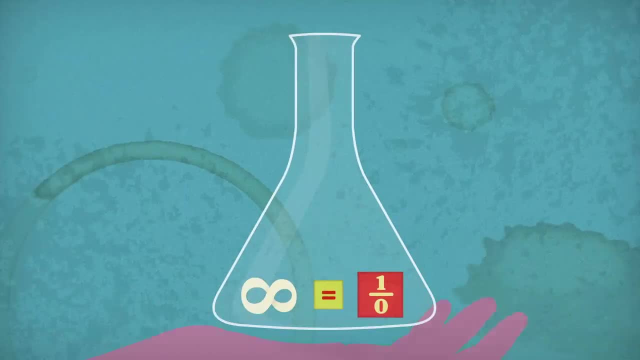 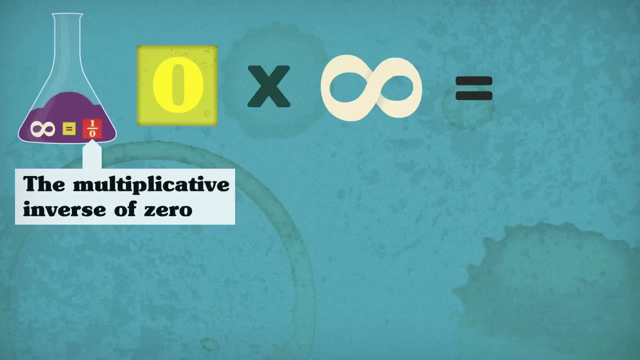 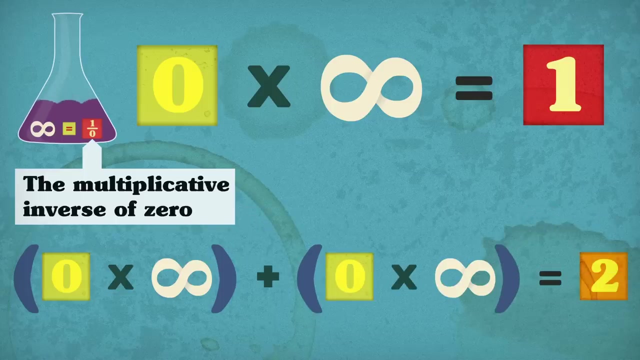 Let's try it, imagining we don't know anything about infinity. already, Based on the definition of a multiplicative inverse, 0 times infinity must be equal to 1.. That means 0 times infinity plus 0 times infinity. Now, by the distributive property, the left side of the equation can be rearranged to: